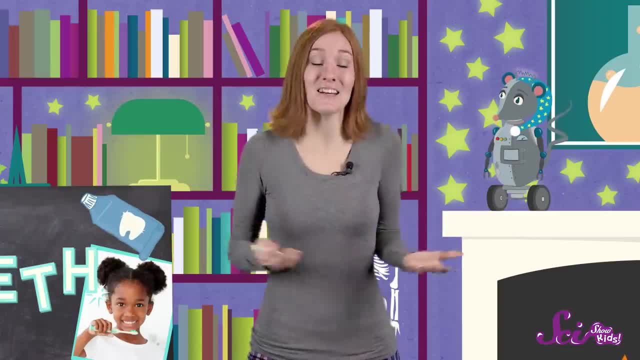 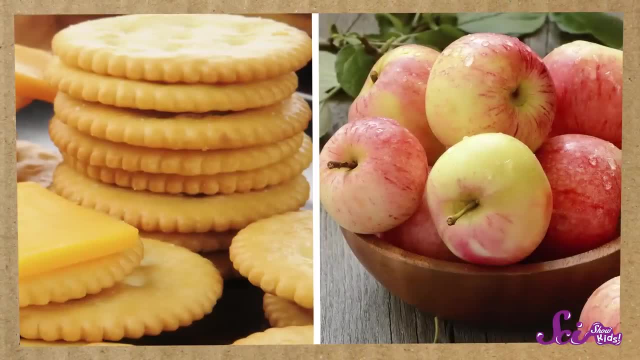 good, because it is good. We brush our teeth to keep them clean and healthy so they can keep helping us our whole lives. After all, how would you crunch up a cracker or bite into an apple without them? Without teeth, you'd have very few choices of foods that you could eat. so you've got. 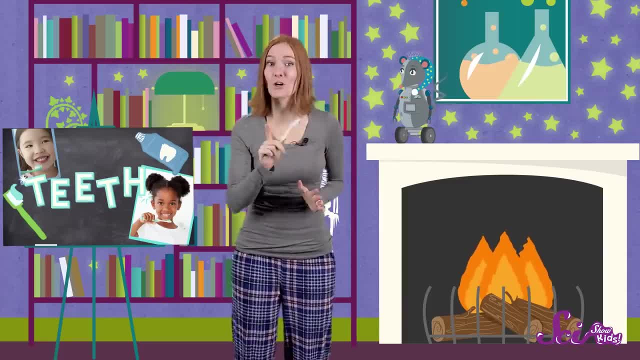 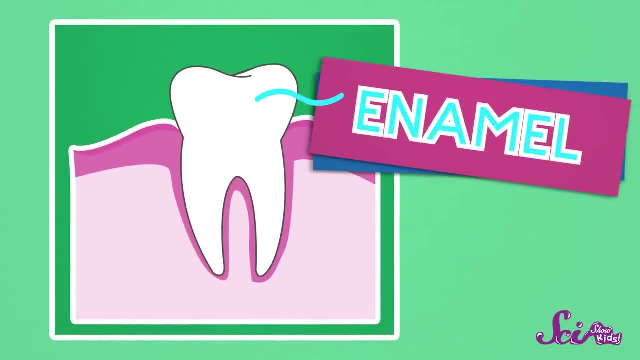 to take care of them. Now, you can't tell by just looking at them, but your teeth are actually made up of different layers. The part that you can see on the outside is a super hard shell called enamel, which is mostly made of minerals. 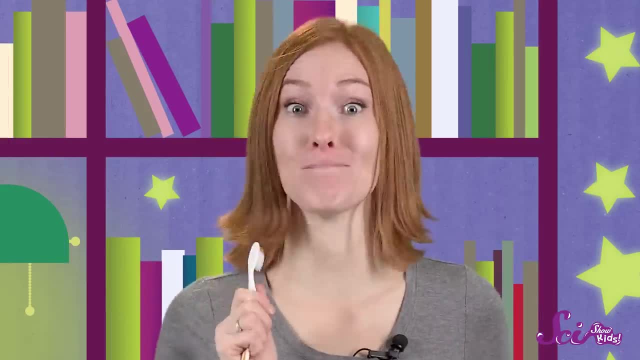 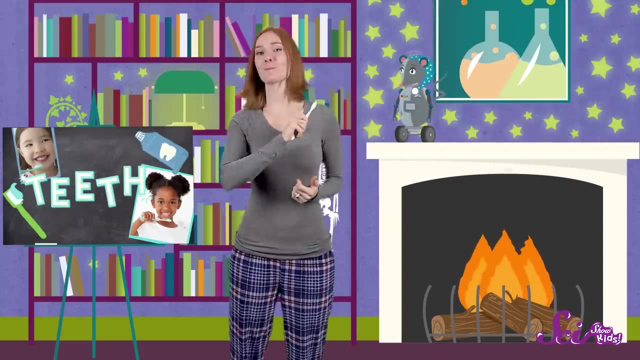 Enamel is the strongest stuff in your whole body, even stronger than bone. But unlike your bones, a tooth can't heal itself if it's broken, And your teeth are not hard enamel all the way through. Just below that tough outer layer there's another layer called dentin. that's not as 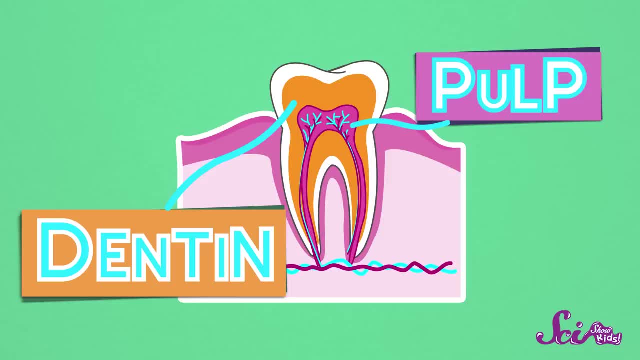 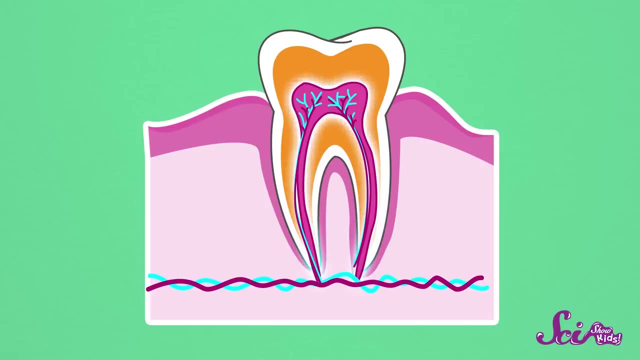 hard, And below that there's the inner layer of the tooth, called the pulp, which has blood vessels and nerves inside it, And this part of your tooth is super sensitive. So in order to protect the delicate pulp inside of your teeth, you have to take really 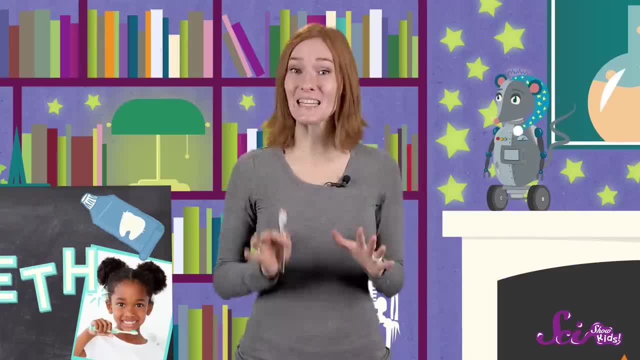 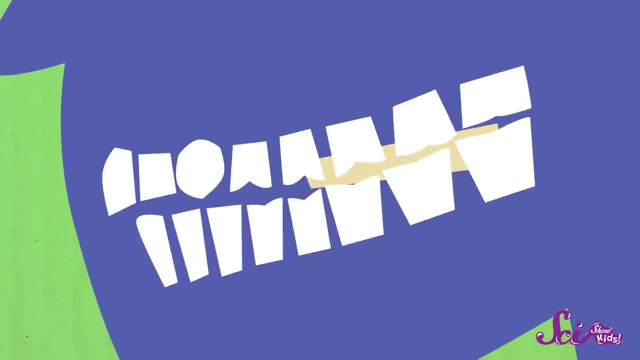 good care of the outside, And the best way to do that is to clean them up after you eat, Because food can damage even those tough outer layers of your teeth. How Well you might think that you ate every last bite of those crackers you had for a snack. 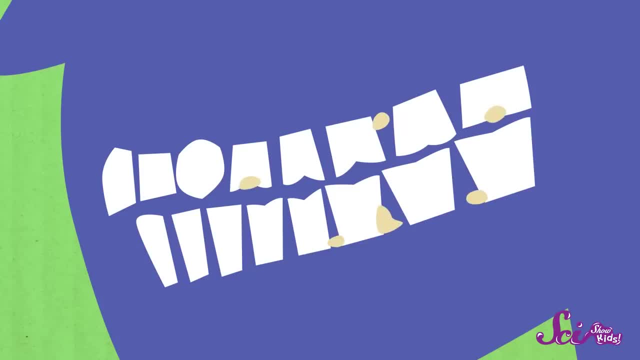 But the truth is, some very small pieces of food are still hanging around in your teeth. That's because your teeth aren't all shiny and smooth. They have lots of bumps and ridges that help you grind down your food And there are lots of small spots on your teeth. 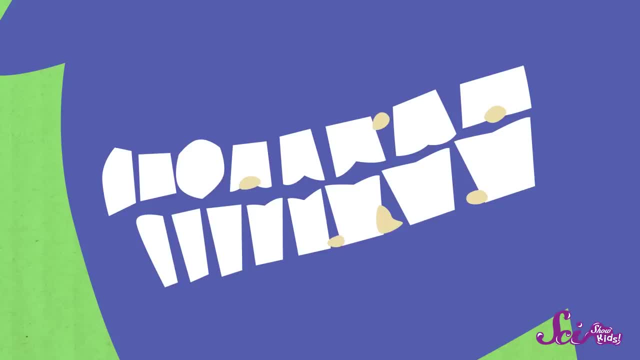 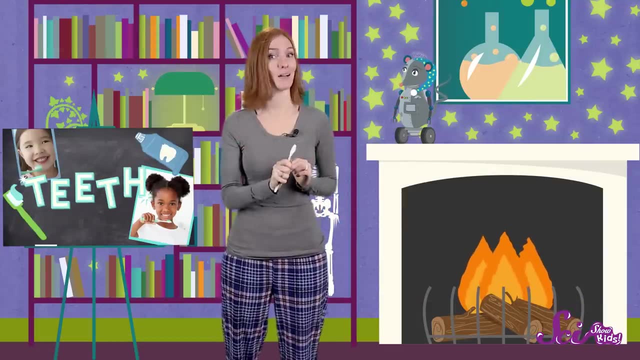 And there are lots of small spaces between them too. These are places where it's easy for food to get stuck and hang out all day, Which is kind of gross. But you know what's even more gross? You're not the only one enjoying these leftovers. 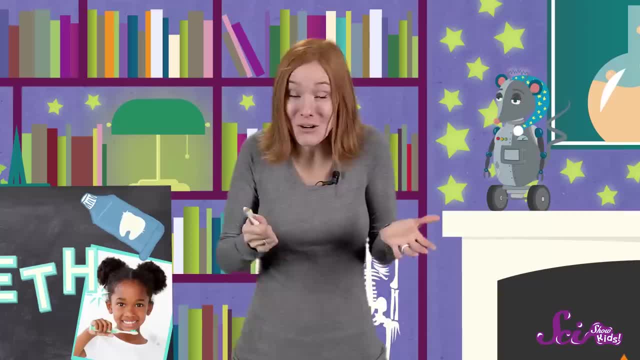 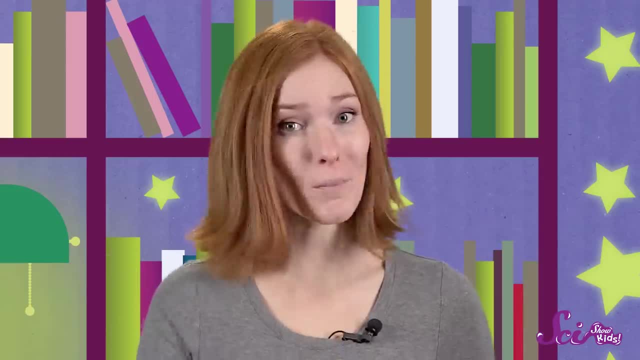 There are lots of tiny little things that call your mouth home. These are called bacteria. They're way too small to see, but they're definitely in there, And there are a lot of them In just your mouth alone. there are more bacteria than there are people on Earth. Some kinds of bacteria are really good to have Bacteria just kind of hang around and are neither good nor bad. And then there are some who are pretty bad houseguests and you don't want them staying in your mouth for too long. One type of bacteria loves to eat the same stuff that you do, especially sugars and starches. That means things like cookies, chips, bread, candy and cereal. These bacteria hang around on your teeth and in your mouth, basically eating your leftovers. 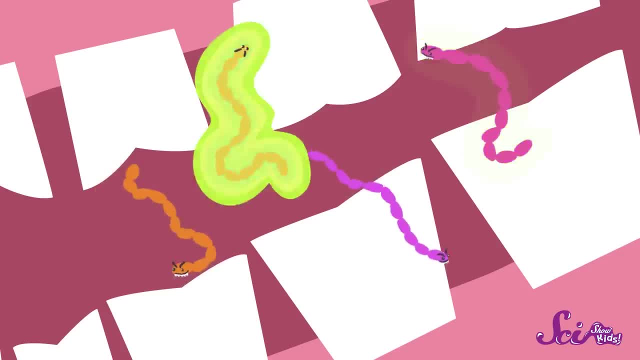 And once they're done eating those tiny bits of food, they release acid which can really hurt your teeth. This acid can cause holes called cavities to form in the enamel. They're called cavities. They're called cavities.